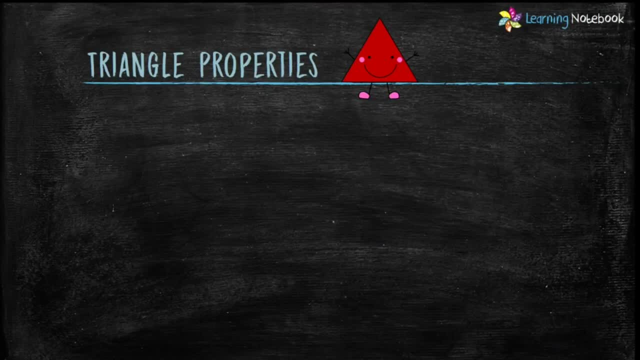 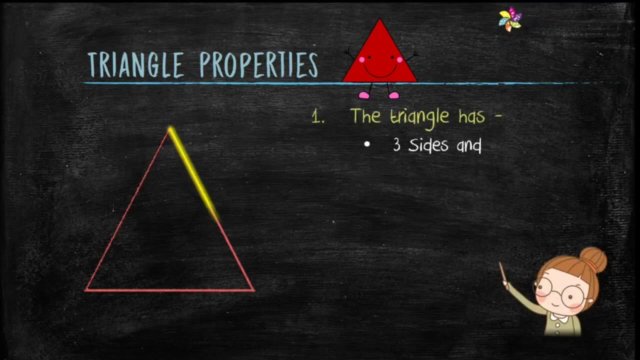 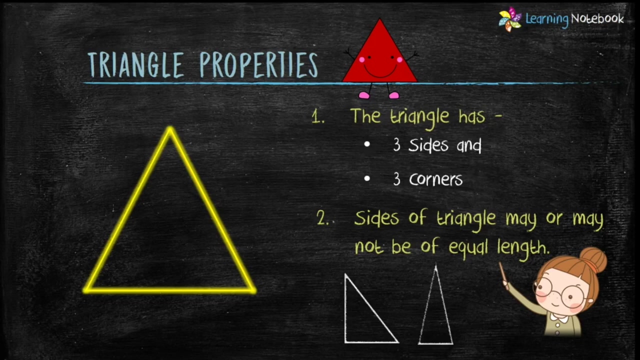 of square. Next basic shape is triangle. First property of a triangle is that it has three sides and three corners, But please note that sides of triangle may or may not be of equal length, like shown in the examples below. Let's see some examples of triangle. A pizza slice. 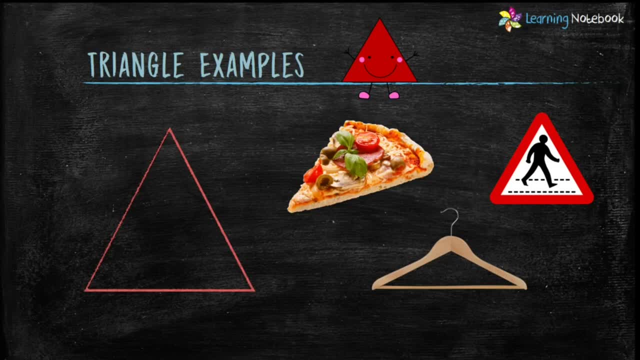 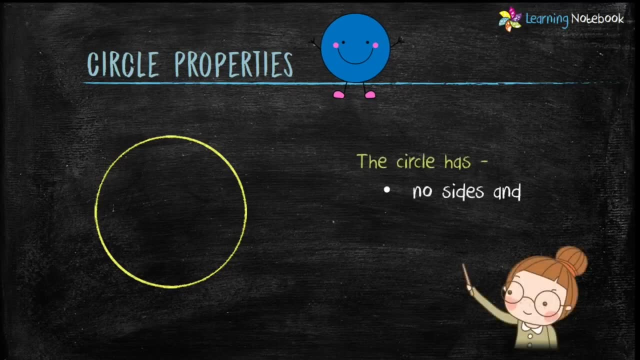 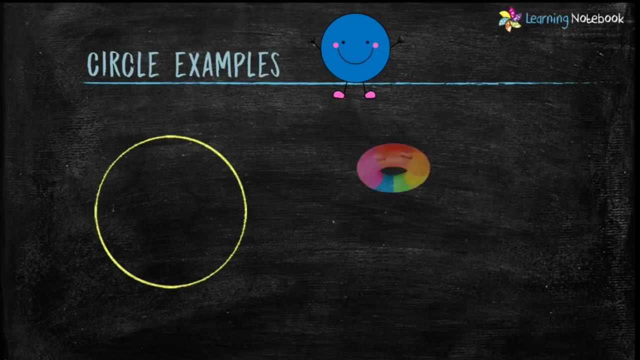 road signs and a hanger. These are examples of triangle. Let's see some examples of triangle. These all are triangle in shape. Last basic shape is a circle. A circle has no sides and no corners. Some examples of circle are shape of a swimming tube, shape of a button and surface of a coin. 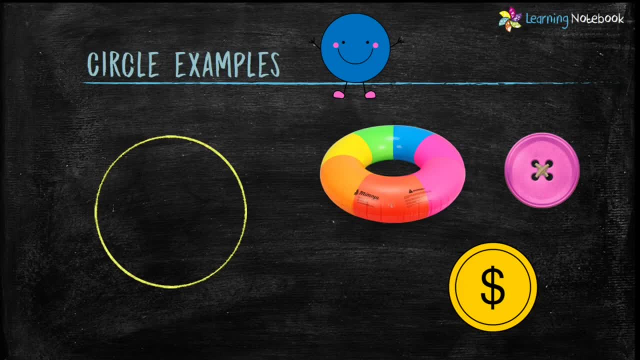 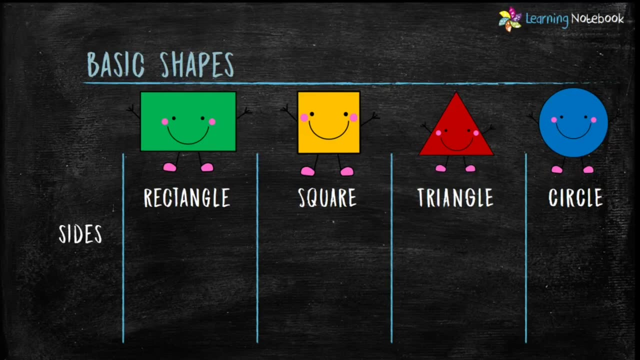 These all are examples of circle. Students, let's summarize what we have learnt so far. Both rectangle and square have four sides. Triangle has three sides, while circle has no side. Then both rectangle and square have four corners. Triangle has three corners and circle has no corner. 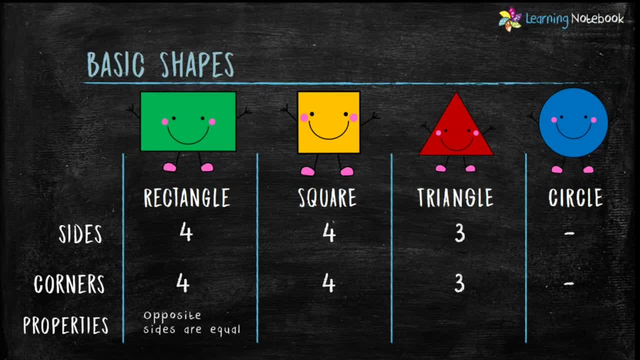 Opposite sides of a rectangle are equal, While all sides of square are equal and, as we have seen earlier, sides of a triangle may or may not be equal, and for circle, we know it does not have any side. Let's do some exercise related to these basic shapes. 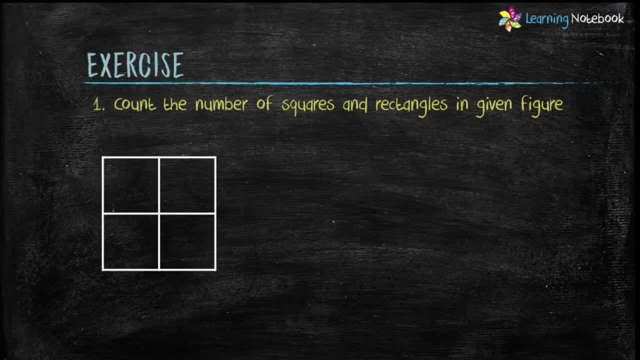 Question is: count the number of squares and rectangles in the given figure? Let's count the number of squares first. Start with the smaller squares. This is square number 1,, 2,, 3,, 4 and 5 is a big square. 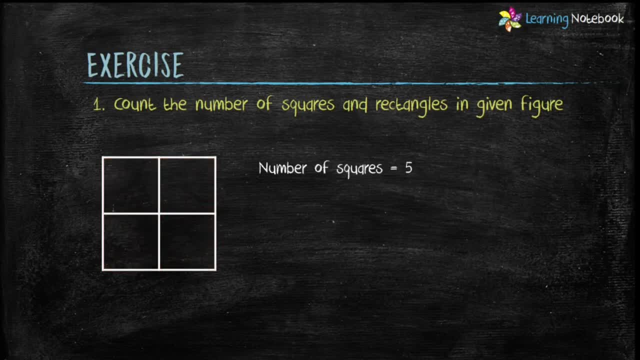 Therefore, number of squares in the given figure equals to 5.. Now let's count the number of rectangles. This is rectangle number 1, 2,, 3 and 4.. Therefore, number of rectangles in the given figure equals to 4..